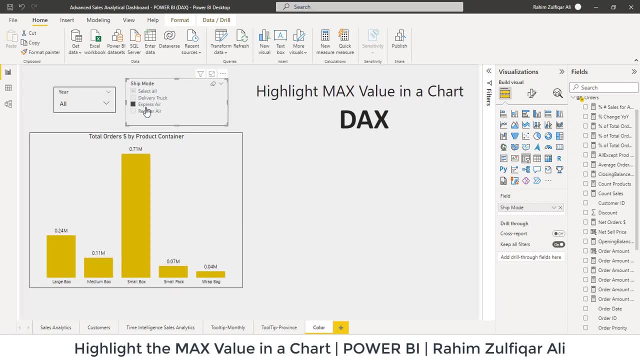 if I select any specific shipping mode, the chart gets changed as of filter context And what we are required to do is, when ever we play with the slicers or we are seeing the overall position, the maximum bar of this, of the particular column, which is the max, should be highlighted with a different color. 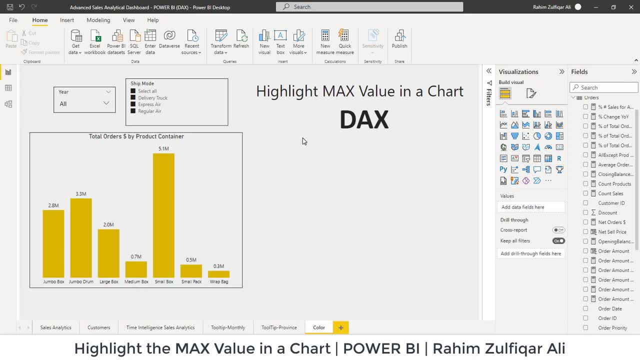 Okay, so for doing that, we are required to create an explicit measure And in that explicit measure we will be defining a variable And we will use that explicit measure in the conditional formatting. So how are we going to do that, How to create that logic? 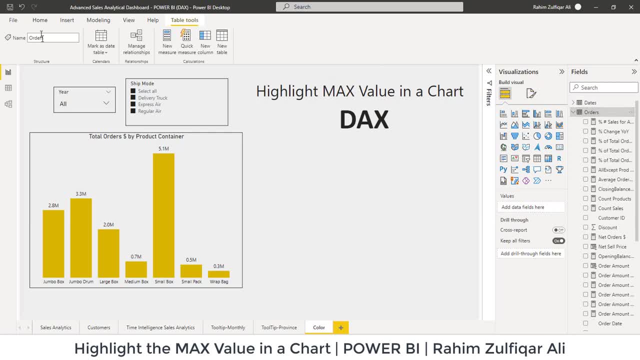 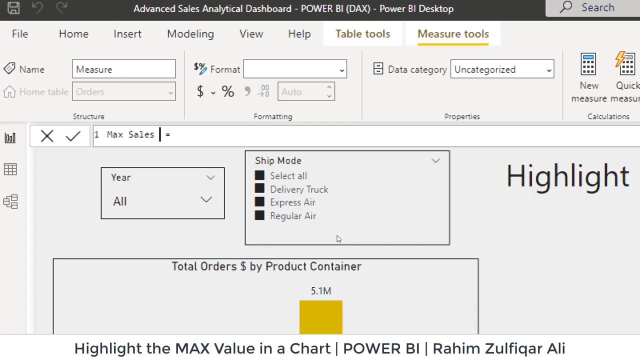 Let's start. So I will go to the home tab And I will click on new measure. So first I need to define the name of the measure. So let's start that. So the name of the measure is: let's give as max sales CF. So I will be using this explicit measure in the conditional. 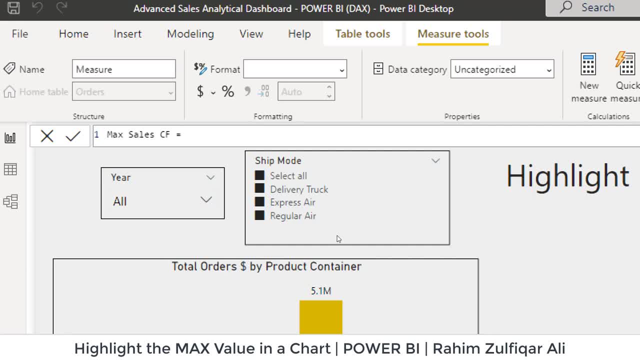 formatting. So starting with first, I will define the name, which is variable. So I will define this variable in the next line. So to move to the next line we have to press ALT Enter key together, So variable, then name of the variable, let's say max sales. 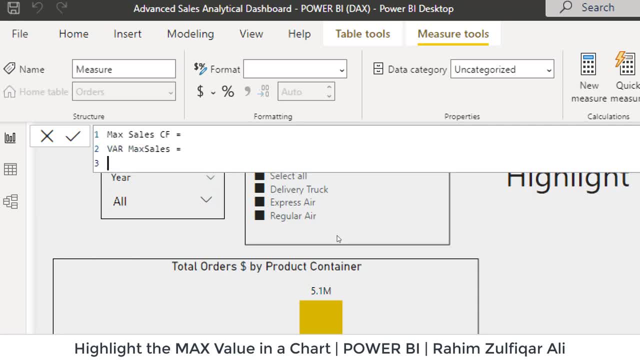 okay, then equals to again, let's go to the next line. The purpose of going to the next line again and again is to make sure that whatever the logic we are creating should be easy, readable and understandable for the other users. Okay, so we are going to start. 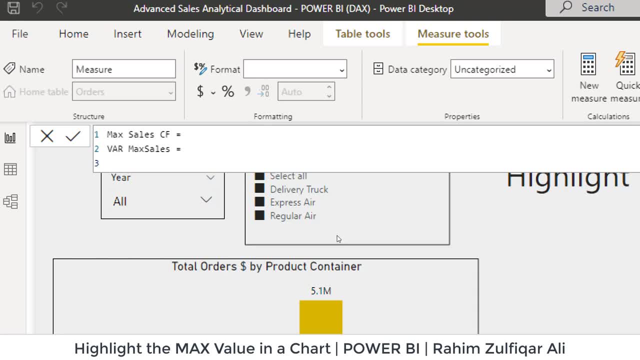 that. So okay. so in the description, for example, I would say: let's say max sales, other users as well. otherwise it will contains a very long one raw in which all different DAXs will go together and sometimes users get confused. so that's why I am putting all the new DAXs into 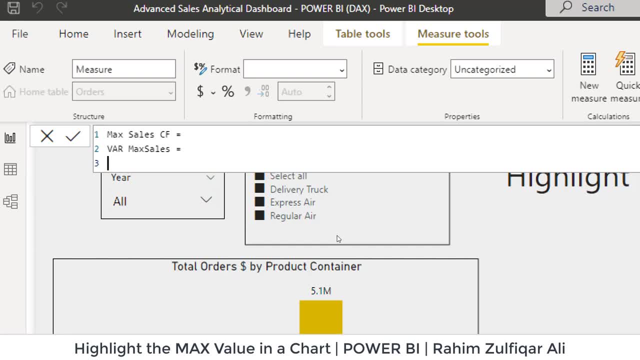 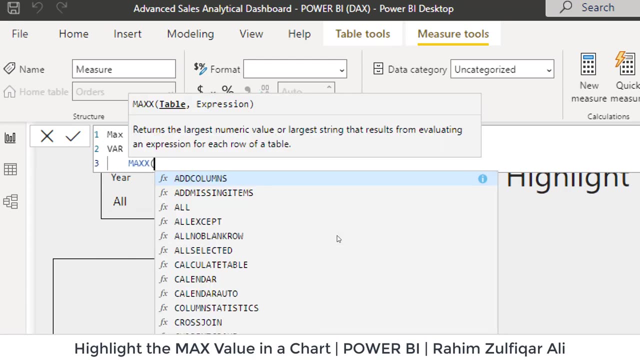 new lines. okay. so first we are defining a variable and the name of the variable is max sales equals to. moving to the next line. I will press the tab key here I will add one DAX which is called max X. okay, and the first argument is the name of the table and then the expression. so in the table, what? 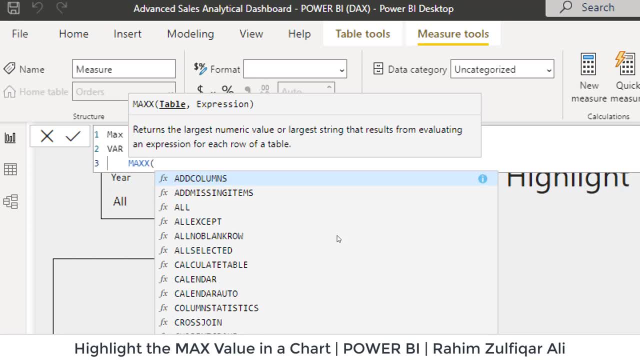 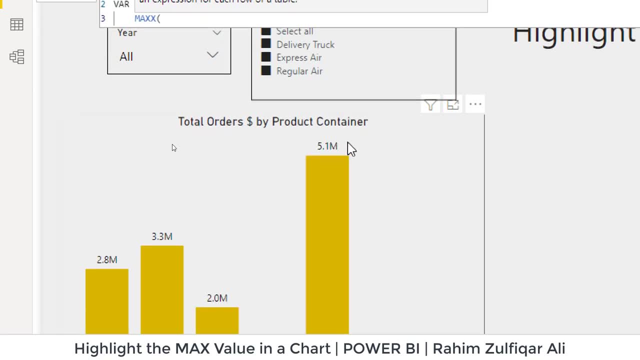 we are going to do is we will be using another DAX, which is the all, to remove all the filters from this particular visual. so, as you can see, that whenever we select any slicer or anything, we do change in our this particular dashboard. so what we need to do is to find a particular 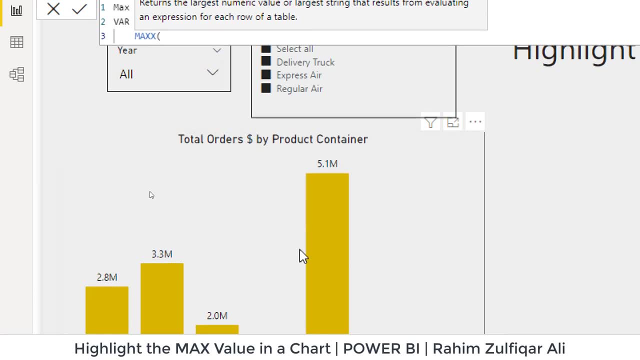 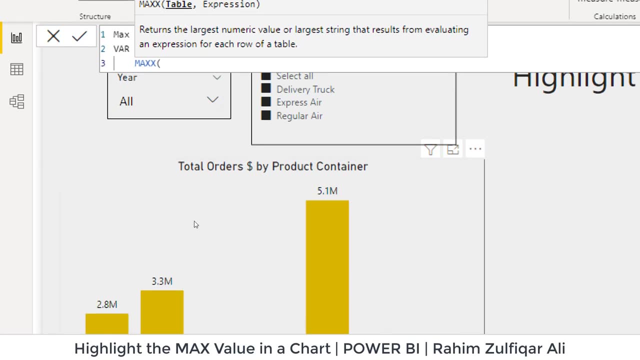 seller or need to change the nom of that seller. we want some one $ rep валenta. that sl�� to know to do is we need to just get rid of the filter thing and we are creating a logic that that we need to remove that filter from the product container. okay, so in this specific column chart, 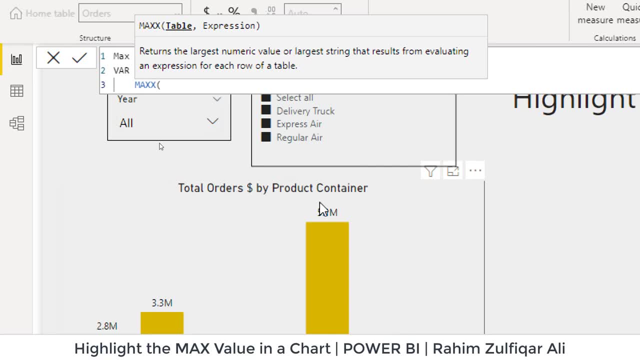 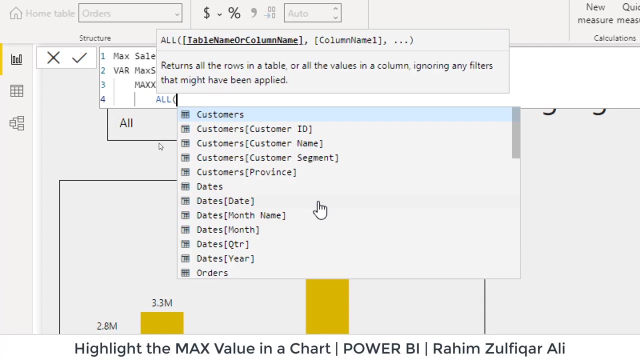 the product container is the field which we are using, so we need to remove the filter uh from that particular visual. so we will be using the all dax, so i will use another line. all bracket open. so from the orders table we have the product container column. okay, bracket close. 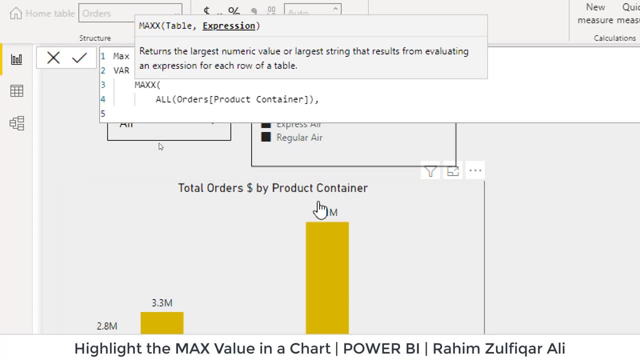 comma. again, let's go to the new line, and here we will be using another explicit measure, which is total orders, that is, the sum of the total orders column in the order stable. okay, and let's go to the next line bracket, close, then again alt enter. now, based on this particular concept, we will add another. 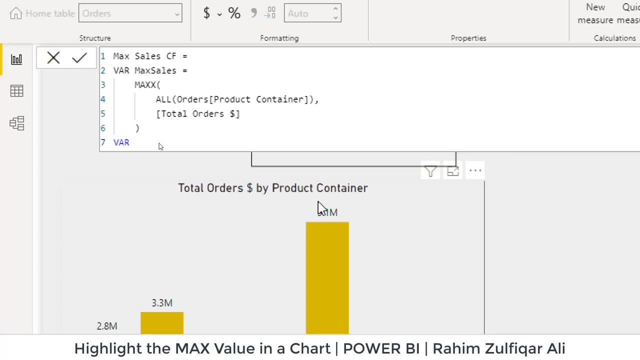 variable, so var, and the name of the variable is the color. so we now we will be defining the color in this particular variable. let's go to the next line. we will be using the if, dax, if bracket open. let's go to the next line. if the total orders is equals to the max sales, which is the 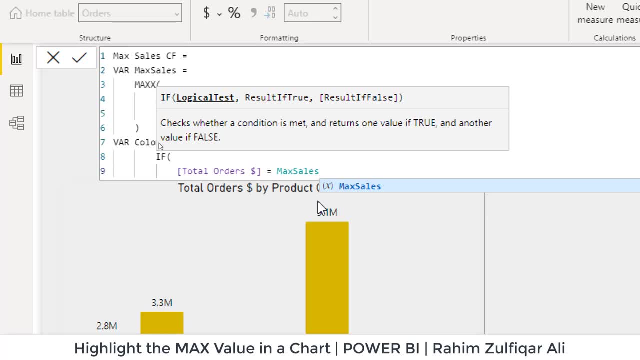 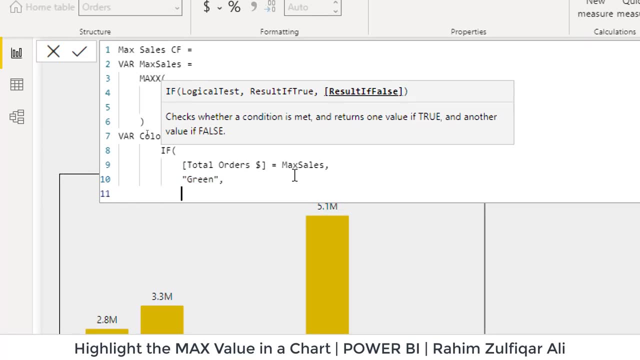 variable, okay, which we have defined just above in the color which is green. so for the remaining, we will define the color which will be dark yellow. okay, and then now we will close the bracket in the next row and after defining the two variables, we need a return. so what? we need a return.